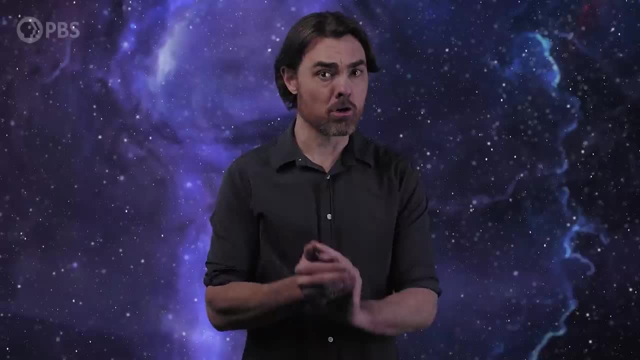 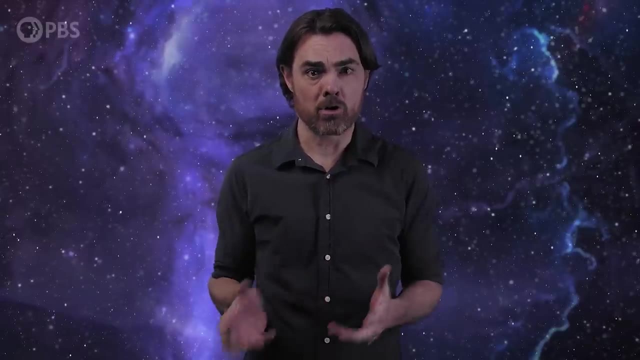 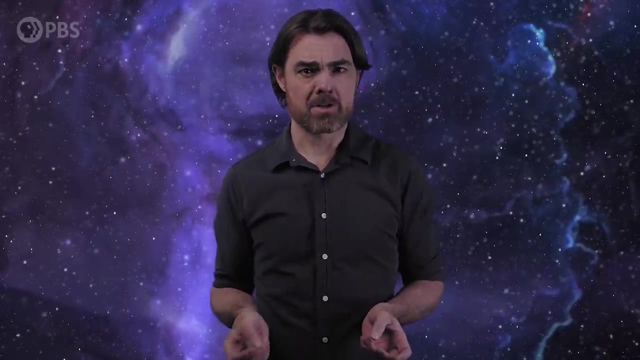 the strong force is entirely confined to the nucleons, and yet somehow it's also the force that binds protons and neutrons together to form most atomic nuclei. That process is strange enough that it deserves its own episode, Especially because it was this very question: how are atomic nuclei held together? 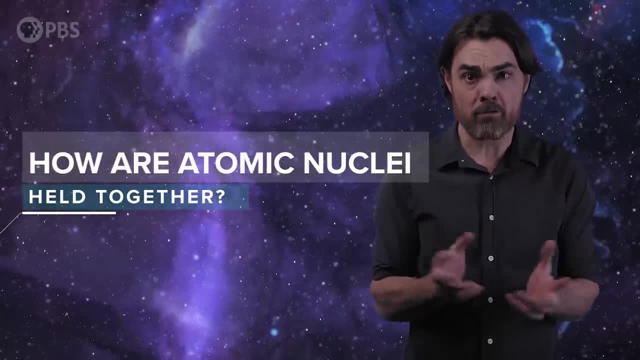 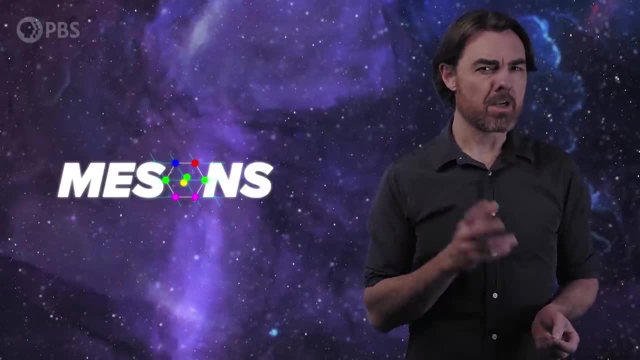 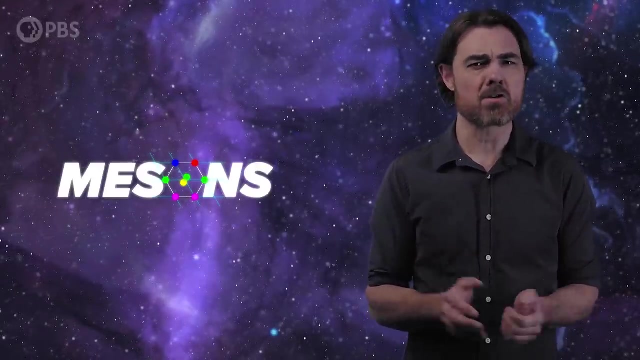 that led to the discovery of both the strong and the weak forces in the first place. But this is also the story of the meson, the obscure cousin of the proton and the neutron that, while less known, is just as essential to the existence of all complex. 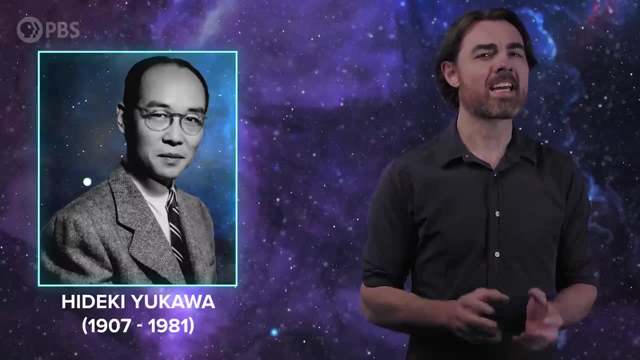 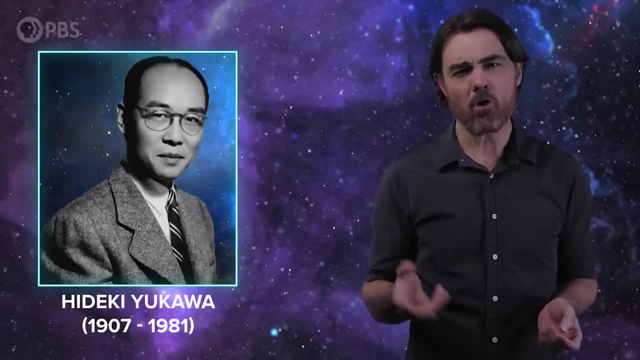 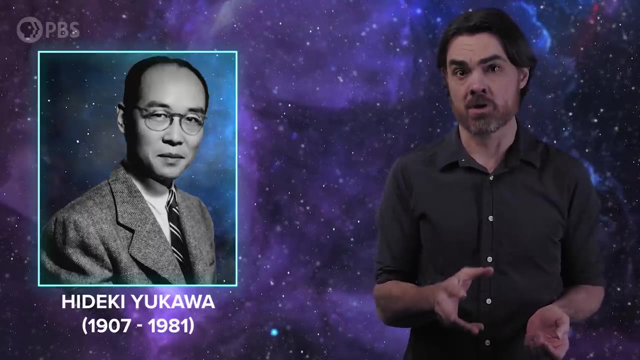 matter in the universe. Our story starts with Hideki Yukawa, a young physicist who graduated from the University of Osaka in 1929 before moving back in with his parents and working for no money as a university assistant Due to the Great Depression. not because he wasn't a great. 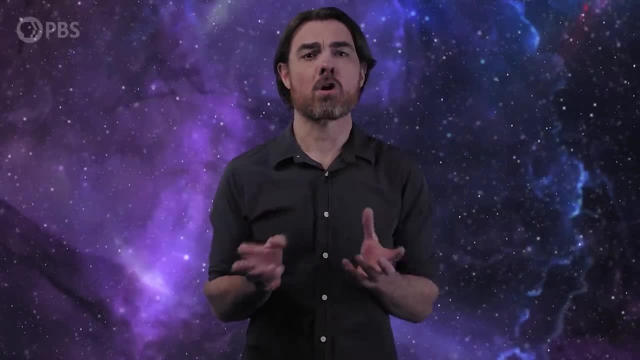 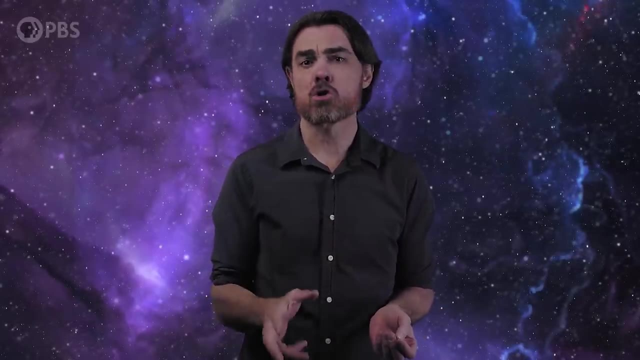 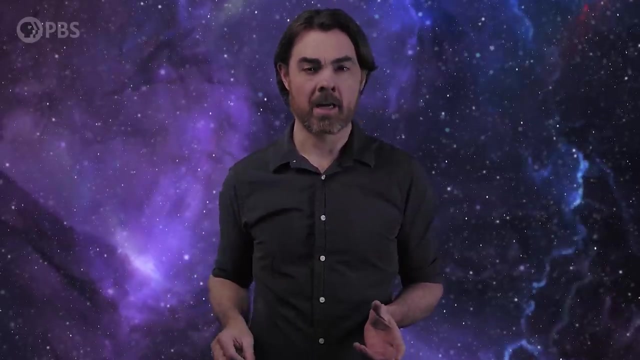 physicist. All the while, Yukawa was focused on the problem of how nucleons stick together, He was perplexed about why a force so strong shouldn't be observable outside atomic nuclei. Yukawa had one intriguing clue to the inner lives of nuclei, and that was 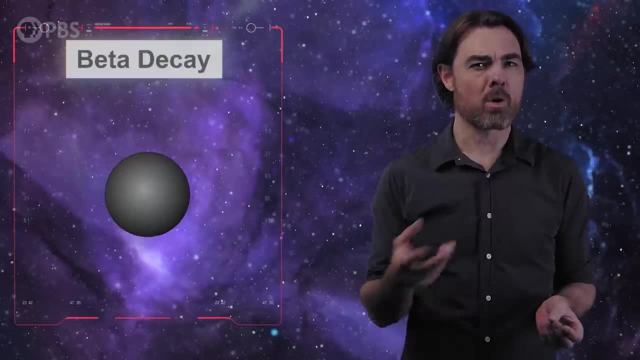 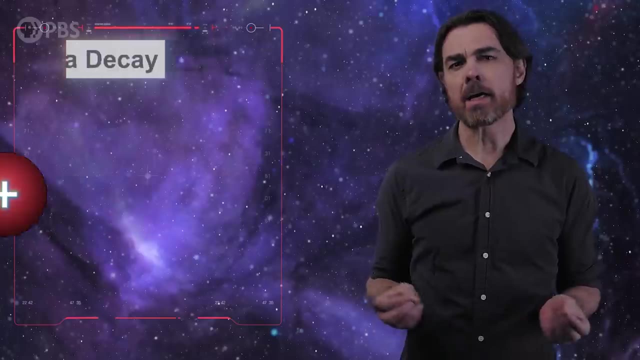 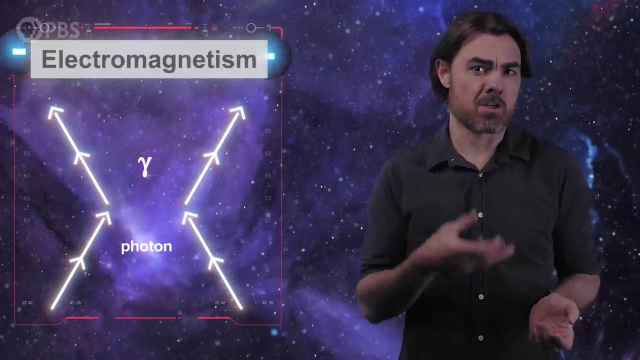 beta decay, The tendency of large nuclei to occasionally spit out an electron and in the process convert one of their neutrons to a proton. He knew that the electromagnetic force is communicated by the exchange of photons, and so it stood to reason that this nuclear force should be mediated by some particle. So what if? 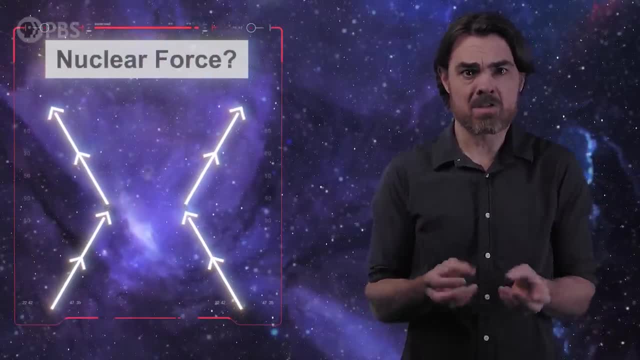 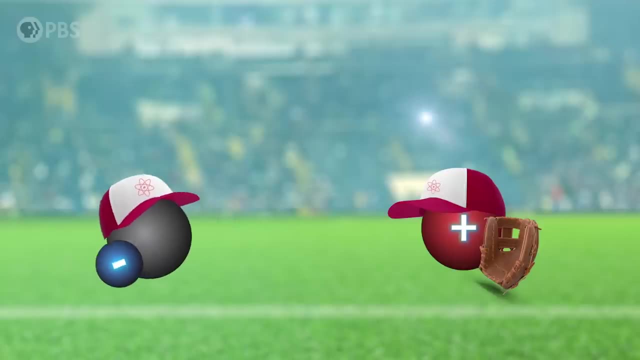 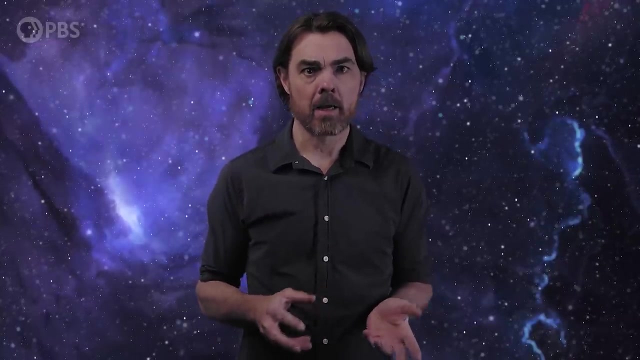 this particle was the electron, and beta decay was the side effect of the exchange of electrons, Like if protons and neutrons were playing catch with the electron, and sometimes they fumbled the ball. It turns out this is totally not what's happening, but the insight that forces should. 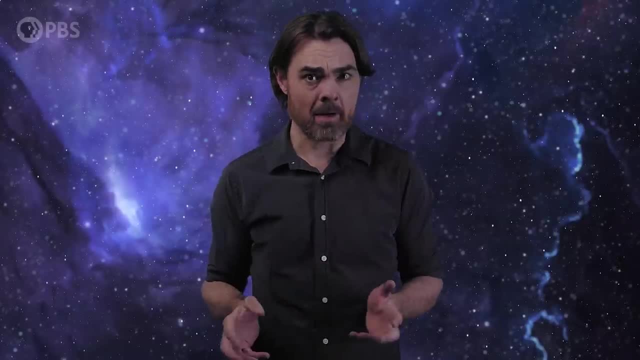 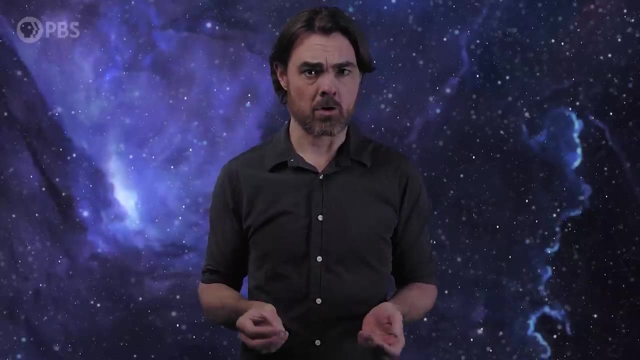 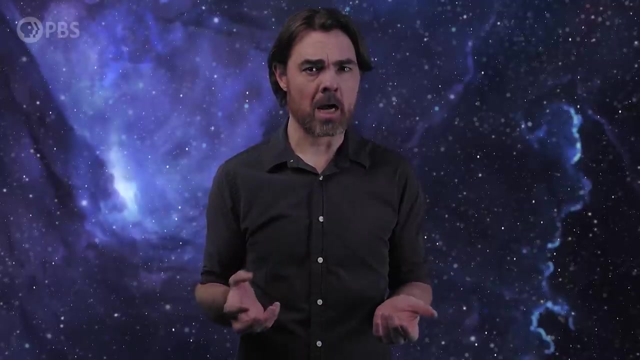 be mediated by a particle was new in its time, and it eventually led Yukawa to the right answer. Having an exchange particle with mass, unlike the massless photon, is a great first step for making a short-range force. These exchange particles are what we call. 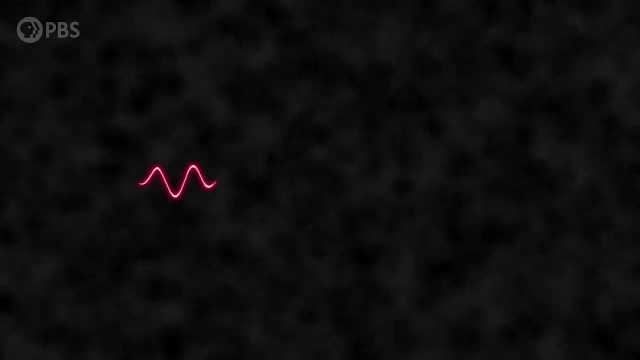 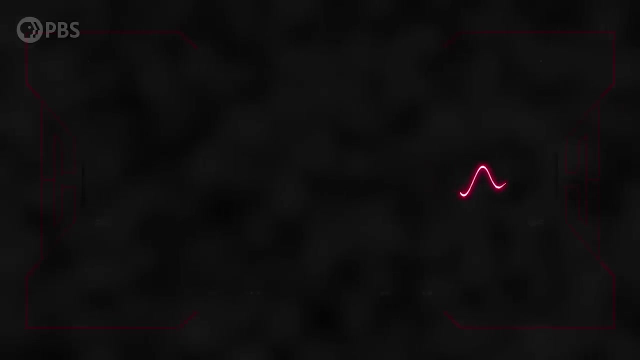 virtual particles, which we've discussed before. Virtual particles can sort of break the laws of physics in the sense that they can pluck the energy needed for their existence out of nowhere, as long as they give it back again. This is a result of the Heisenberg uncertainty principle. 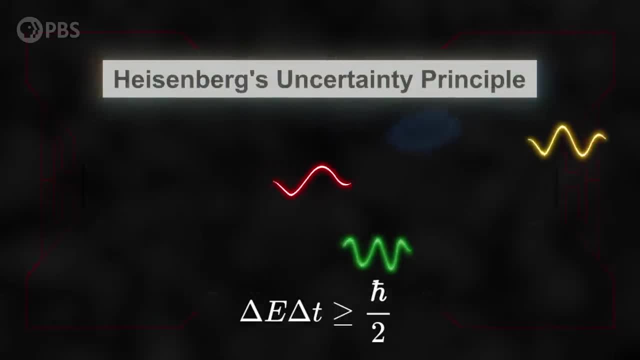 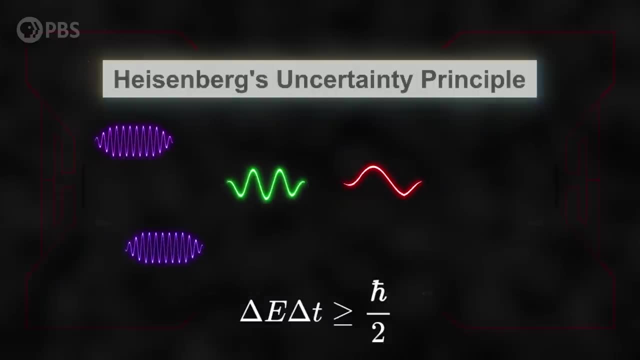 which in one form says that we can never know both the energy and the duration of a phenomenon to better than a certain tiny accuracy. That means, for very short periods of time, the amount of energy in a patchwork of particles will be less than or equal to the amount of energy. 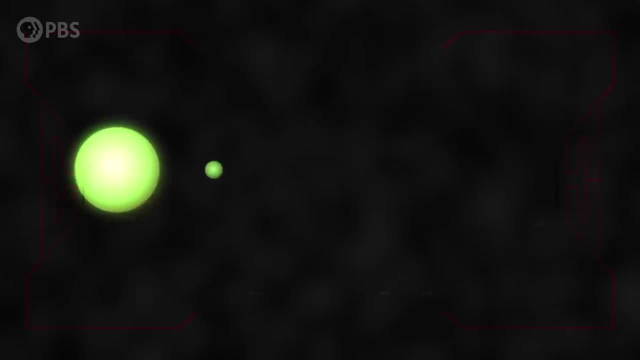 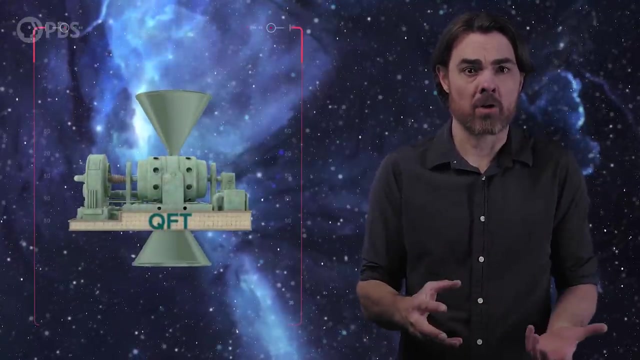 in a patch of space. Mass is a form of energy, so a virtual particle can briefly gain mass from nothing, But the more mass it has, the less time it can exist. Yukawa used the electron mass to calculate the strength and range of a force that could be mediated by the electron, assuming that 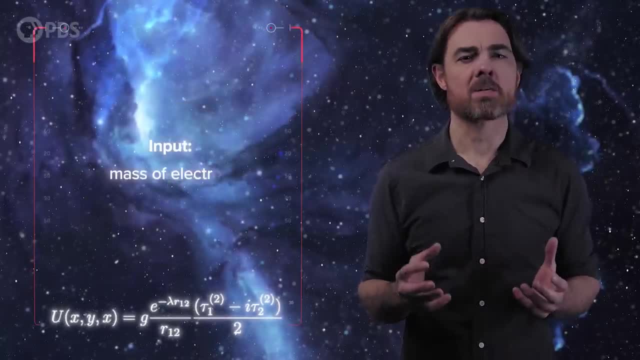 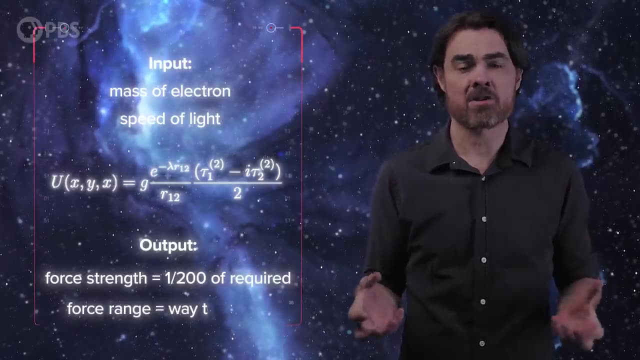 it was traveling at near the speed of light. The resulting force turned out to be around only 1 to 100th of the strength needed to hold the nucleus together, and had a range much larger than the size of the atomic clock. So this is a very interesting way to look at the future of the 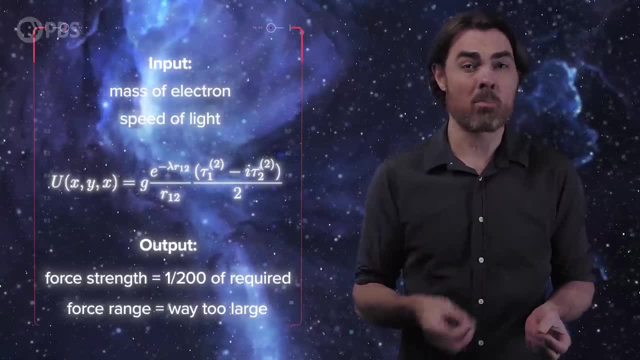 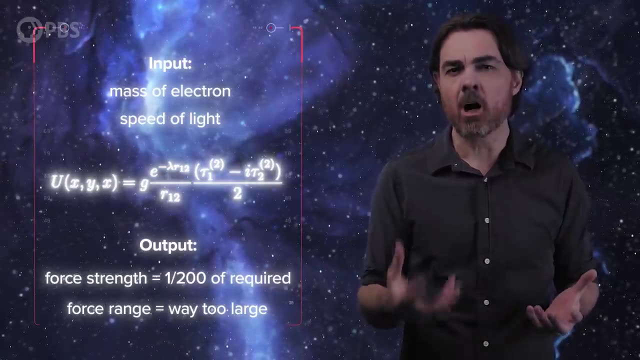 electron. But this is a very interesting way to look at the future of the electron. This is a very make nucleus, so the electron couldn't really be the particle mediating this nuclear force. But Yukawa now had an equation that described the type of force he wanted. 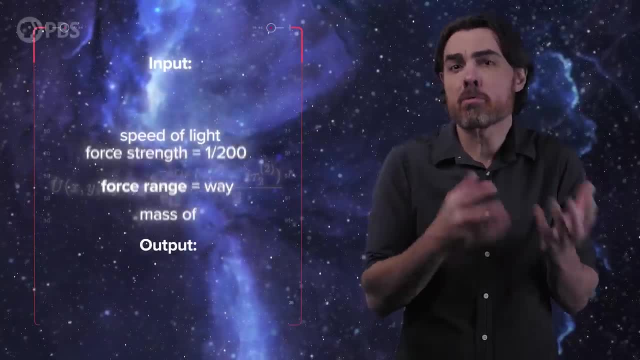 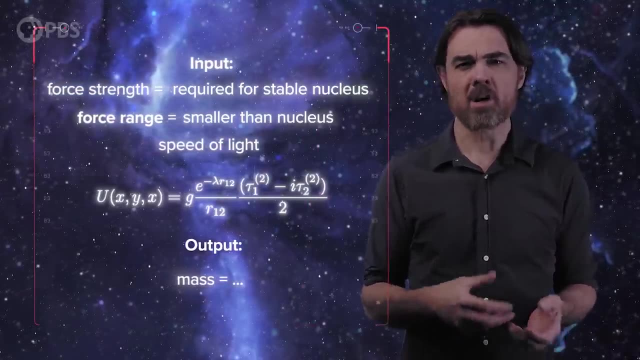 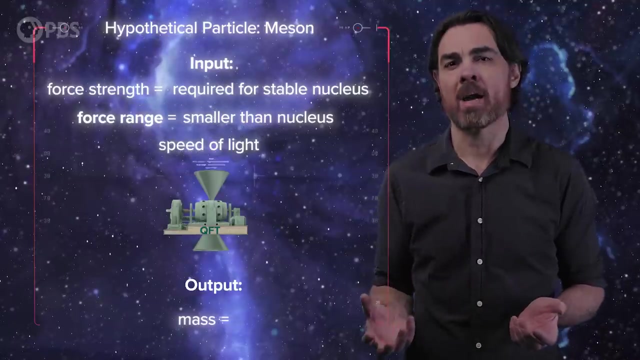 He adjusted the equation to describe a force with the appropriate strength and range and found that it required a much more massive exchange particle. He called this hypothetical particle the meson from the Greek mesos for middle, because it had to have a mass somewhere between the masses. 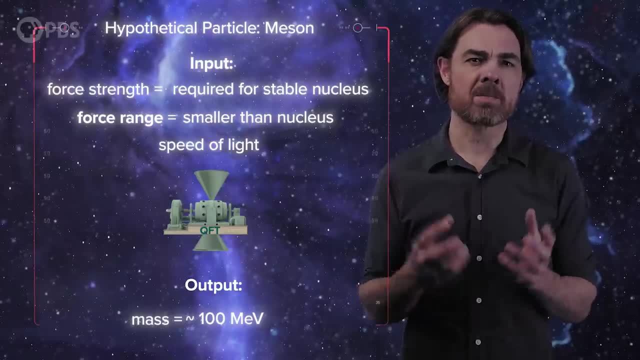 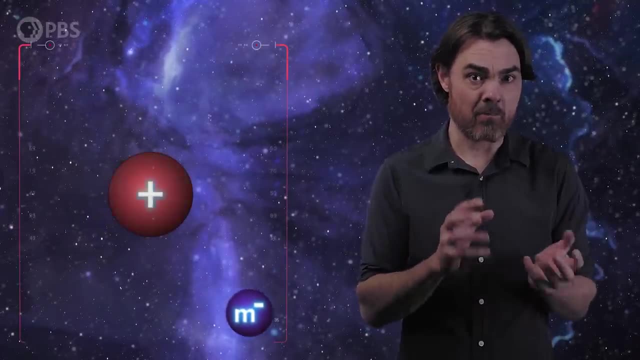 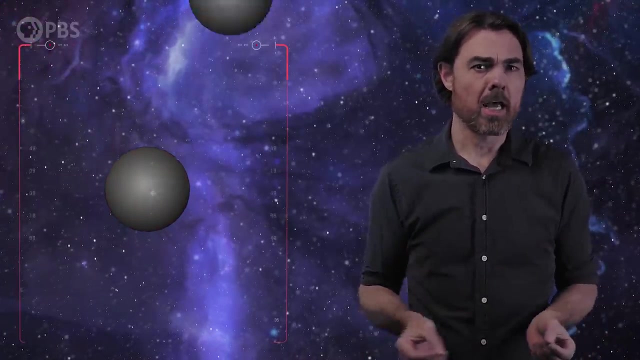 of the proton and the electron. Yukawa also predicted that these particles had to have electric charge. Just like with beta decay: a neutron could emit a negative meson and transform to a proton, or a proton could emit a positive meson and transform to a neutron. 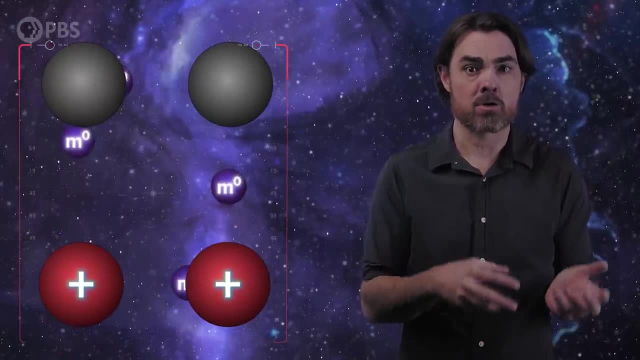 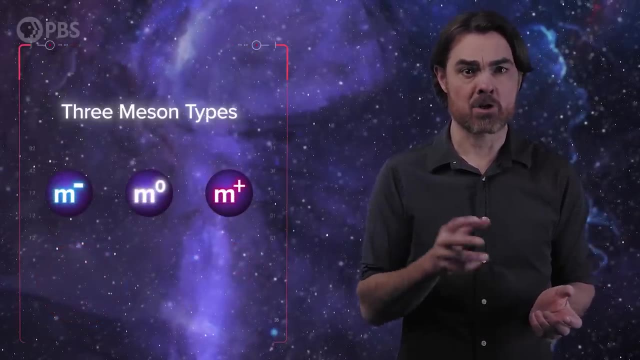 And the neutral meson could be exchanged between protons or between neutrons. As a result, Yukawa predicted three meson types: one for each meson, One for each neutron and one for each neutron. Unfortunately, this new theory didn't explain beta decay at all. 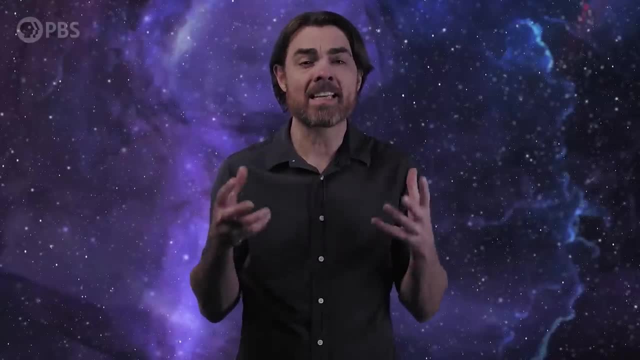 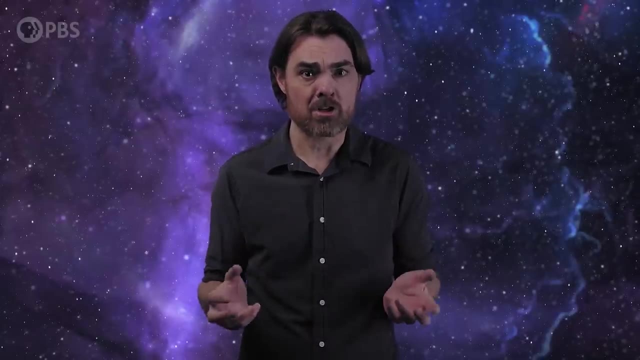 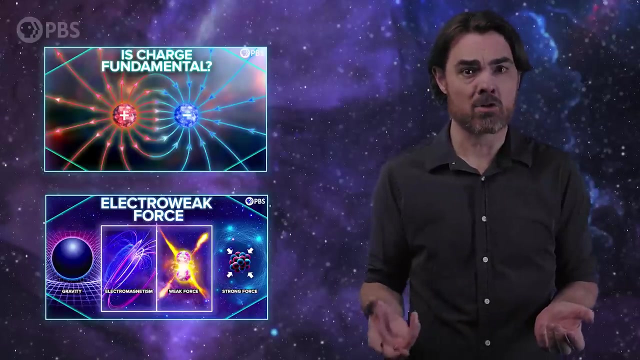 In fact, Yukawa reasoned that beta decay required a completely different nuclear force, much weaker than the one holding the nucleus together. In fact, he correctly predicted the existence of both the strong and the weak forces at the same time, Although the weak force isn't really mediated by electrons. 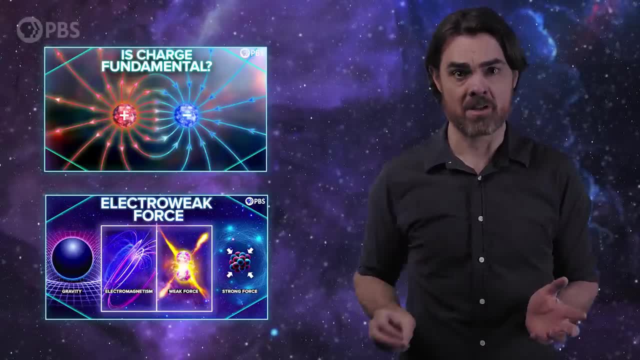 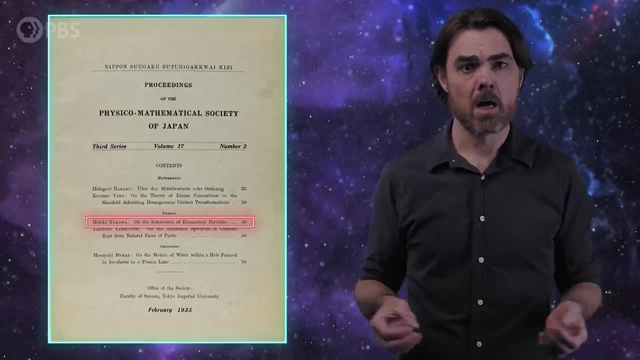 and we have videos explaining everything you probably want to know about it. Yukawa published his theory. He published his theory in 1935, and it was almost completely ignored. To be fair, proposing the existence of two new forces of nature was an extraordinary claim. 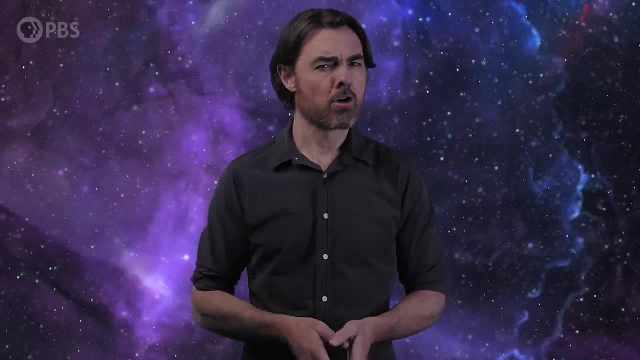 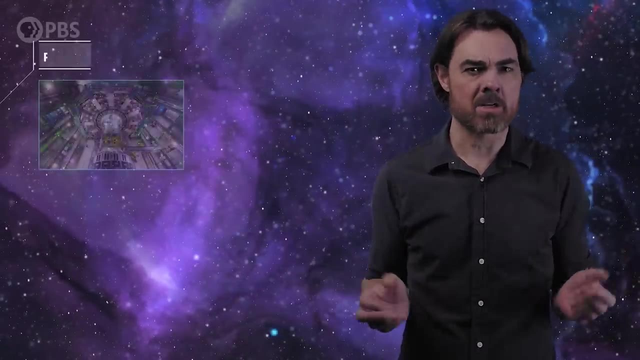 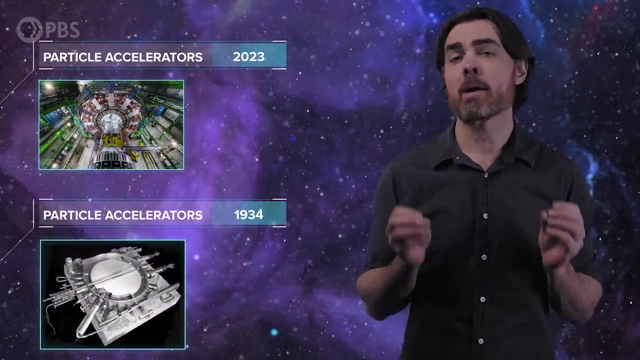 and such claims require extraordinary evidence. No one was going to believe this until we detected a meson. These days, we routinely create countless mesons by smashing atoms together in our particle accelerators. But back then particle accelerators were just being developed, so we had to rely on cosmic light. 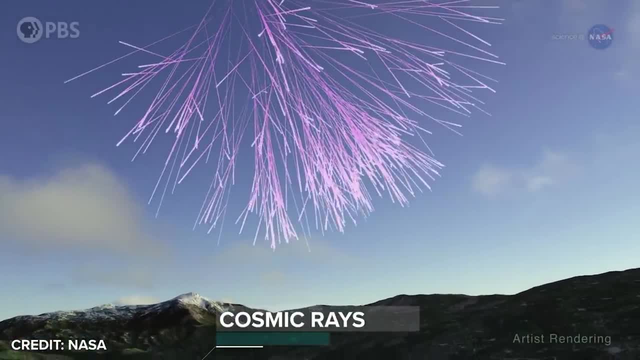 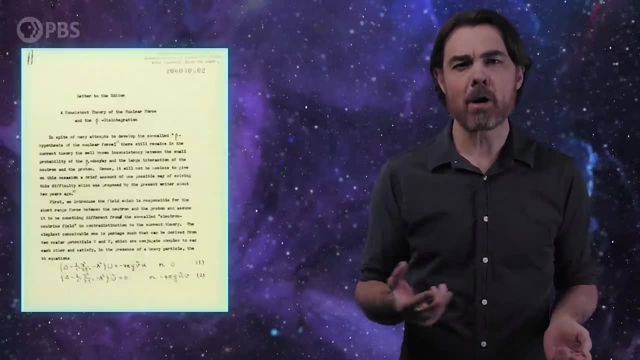 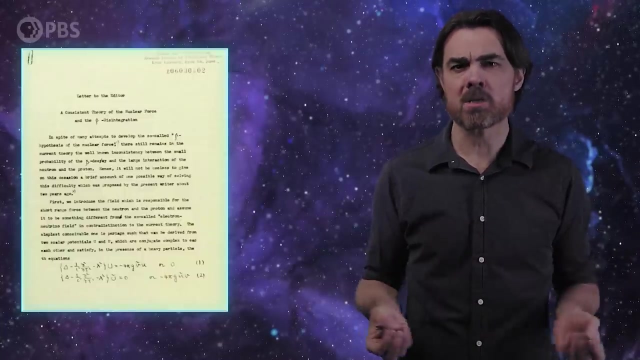 But now we have to rely on cosmic rays. These are high-energy particles that rained down on the Earth from natural space particle accelerators like supernovae and quasars. Yukawa wrote a letter to Nature magazine explaining why cosmic radiation could contain mesons. 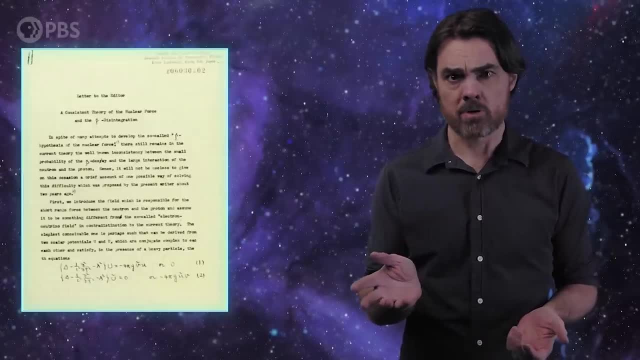 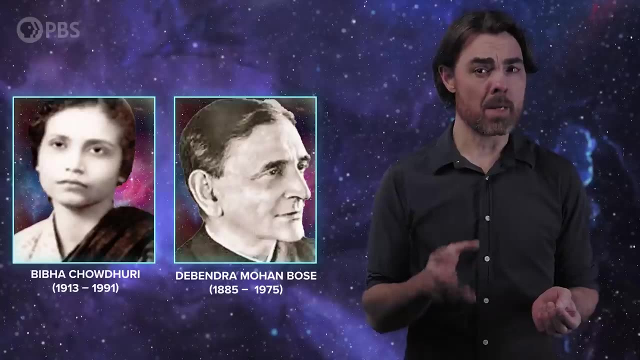 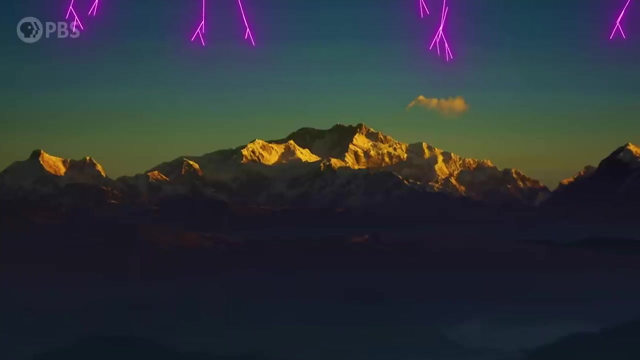 hoping to inspire other researchers to look for these, But his letter was rejected. Nonetheless, others had independently thought of searching for new particles in cosmic radiation- He and Debendra Mohan Bose, for example, who developed a method using photographic plates. They set these up at high altitudes in India and Tibet. 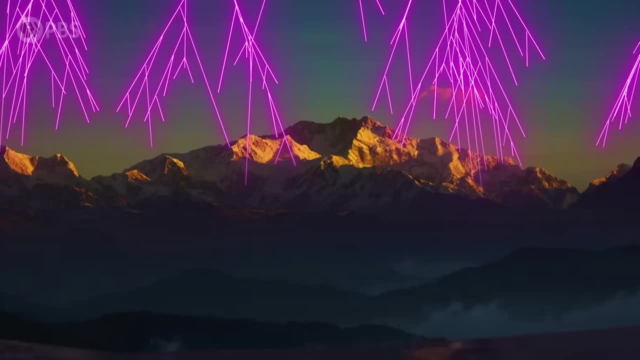 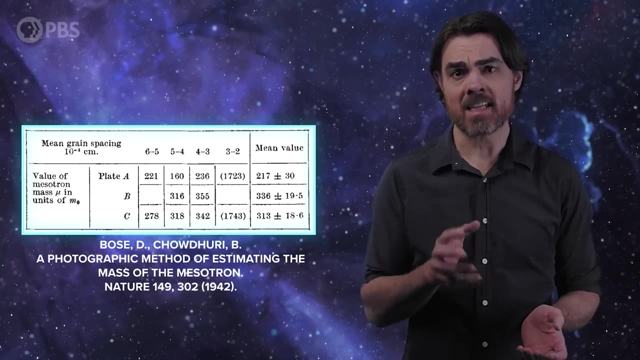 due to the fact that our atmosphere is so good at blocking cosmic rays, which is annoying if you're a particle physicist, but great if you're anyone else. And Chaudhry and Bose did indeed spot the meson at around the mass Yukawa predicted. 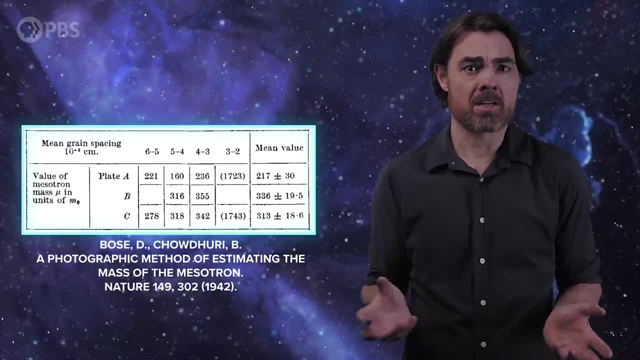 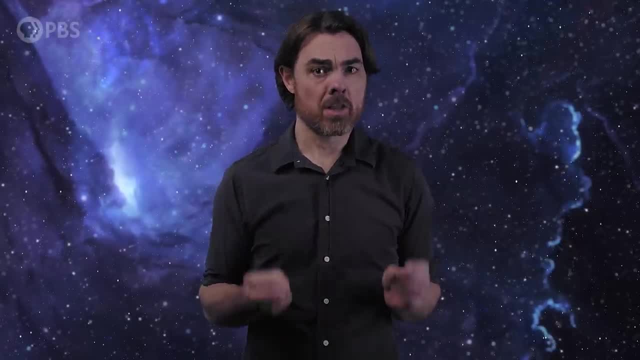 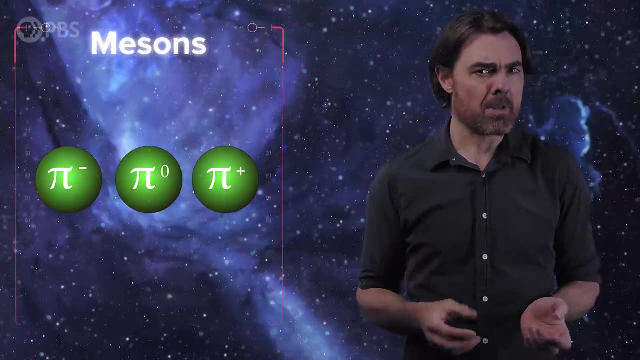 Sadly, their research went mostly unnoticed until British scientists independently found mesons in 1946.. Anyway, not only were these new particles at the right mass range, there were three of them, just as predicted by Yukawa: One positive, one negative and one neutrally charged. 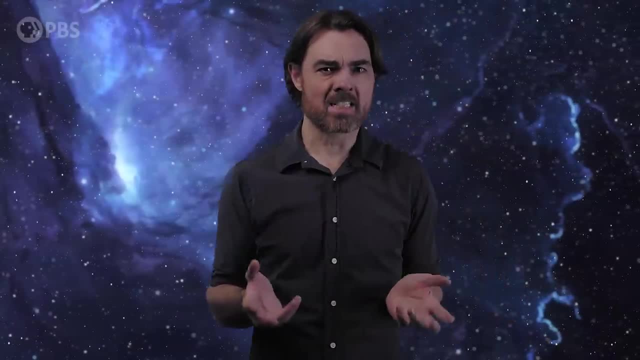 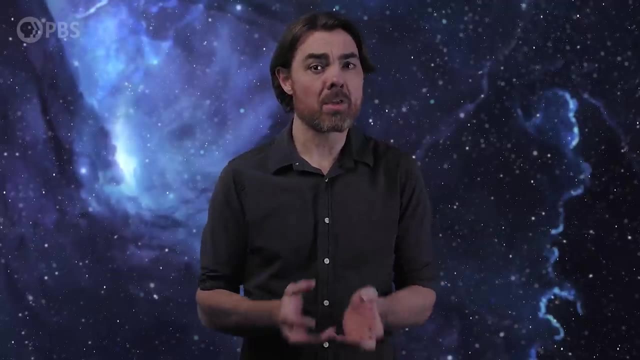 But then things got kind of awkward. Over the next couple of years, thanks to better particle accelerators and improved understanding of radiation, more and more mesons were discovered with a range of properties. The first mesons the ones found by Bose and Chaudhry. 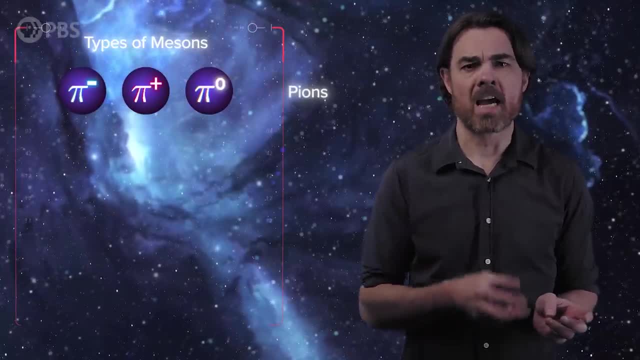 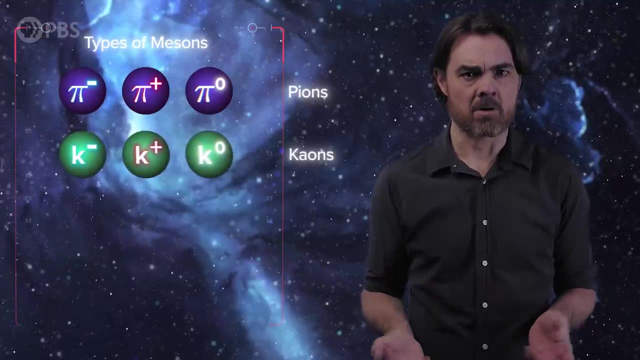 are called pions, And these are the particles actually exchanged by protons and neutrons in the nucleus. But there are many others: Kaons, eta mesons, d mesons, b mesons, et cetera. And to make matters worse, scientists also. 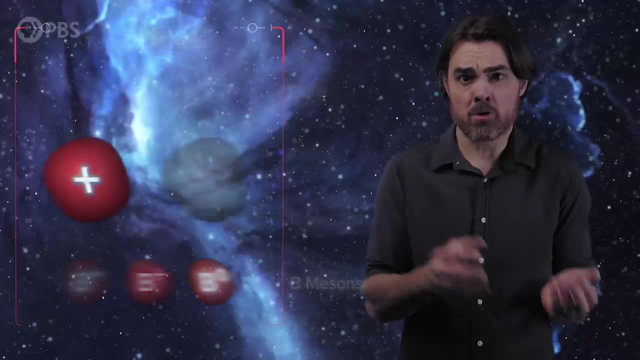 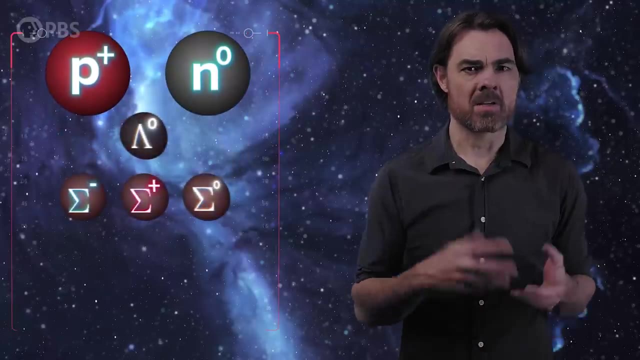 found more particles that could exchange mesons, just like protons and neutrons could. These particles were named baryons, after the Greek word for heavy. There was the lambda, the sigma, the psi, the omega and more. Again, all with different masses charged together. 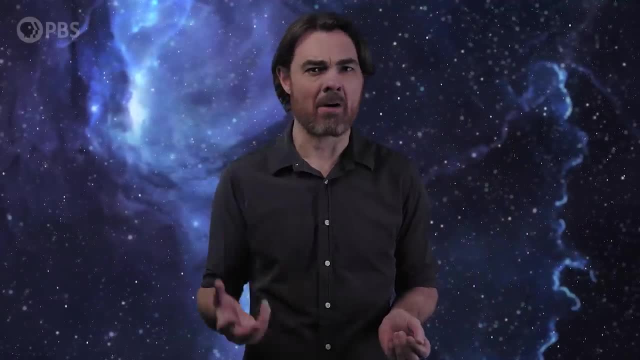 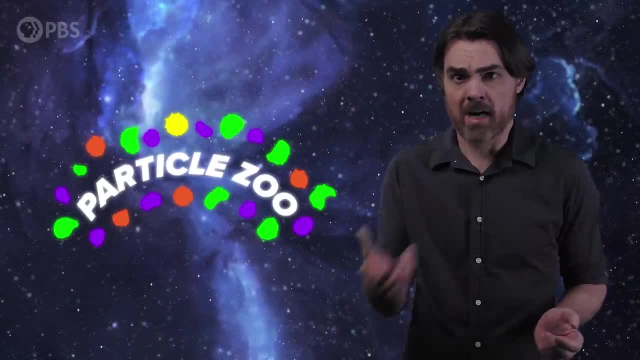 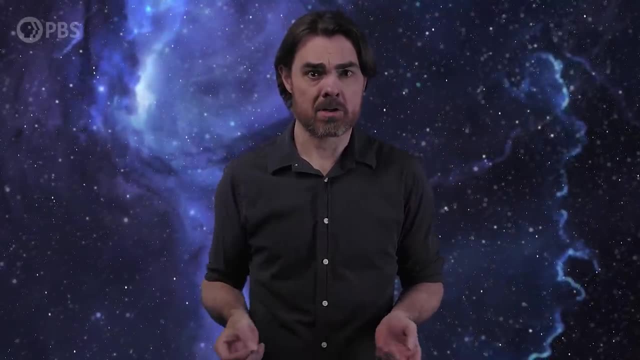 And then there was the particle zoo, And it was a huge problem for physics at the time. According to Yukawa's theory, the atomic nucleus only needs two baryons, the proton and the neutron, and three mesons, the pions. 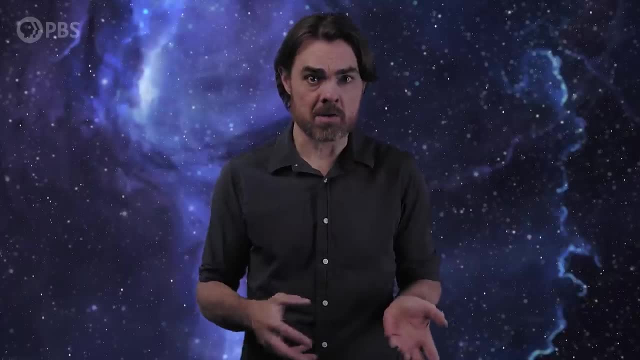 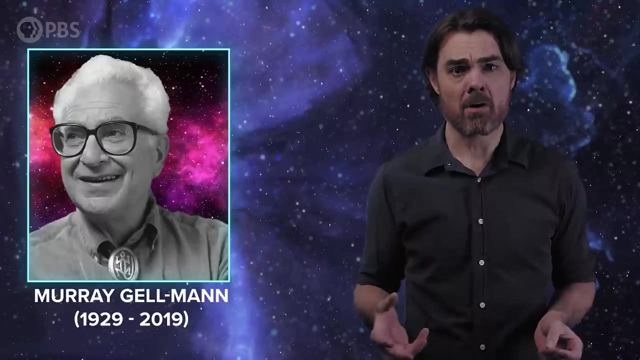 So what was with all of this extra junk that nature doesn't seem to use outside of particle accelerators? This problem was finally solved by Murray Gelman, who realized that mesons and baryons are not the same. They are not elementary particles. 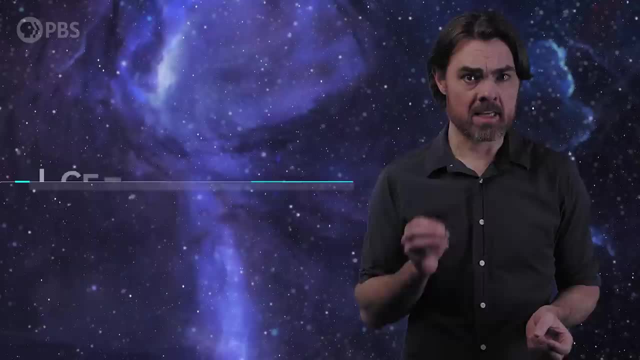 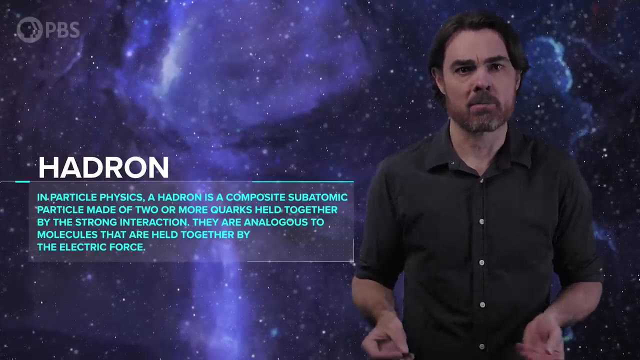 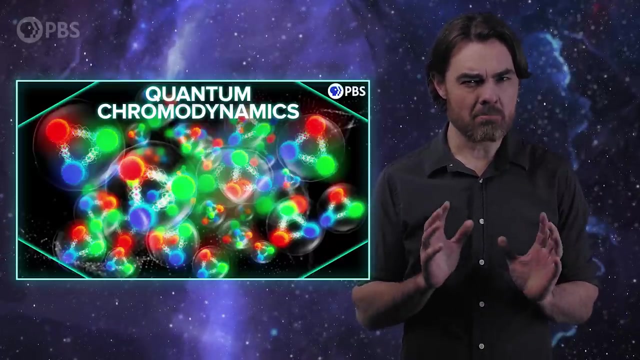 but rather made up of quarks. Hadron is the general name for a particle made of multiple quarks. The particle zoo just results from all the quark combinations that are possible. We covered this in our episode on quantum chromodynamics, but here's a quick refresher so we can get. 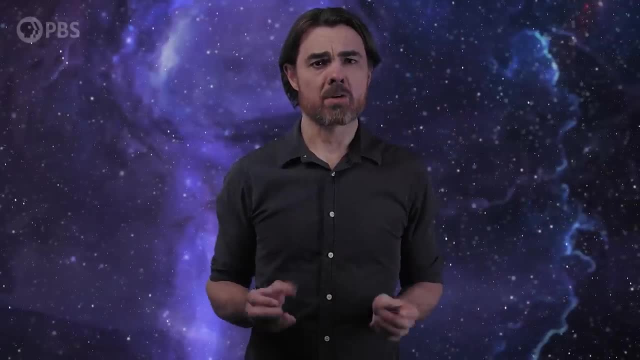 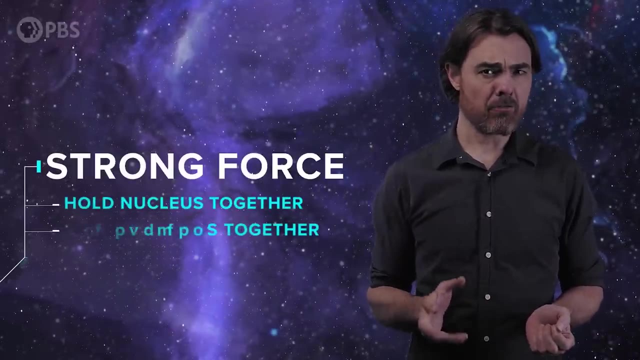 to the punchline of this video. With the discovery of quarks, it was clear that we needed the strong force to not only hold the nucleus together, but also hold nucleons together. In fact, the latter is what the strong force really does. 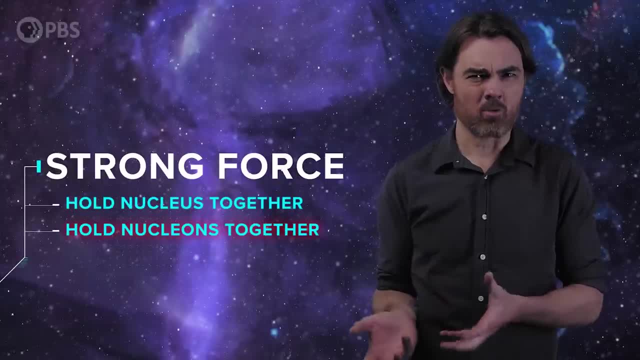 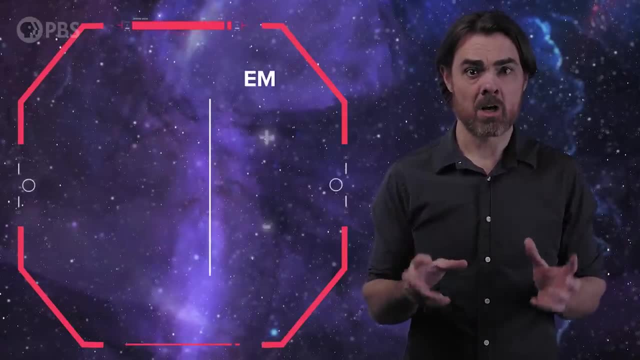 Binding nucleons is sort of an afterthought and not quite directly what the strong force does. So just as electromagnetism works on things with electric charge, the strong force works on things with color charge. There are three types of color charge. 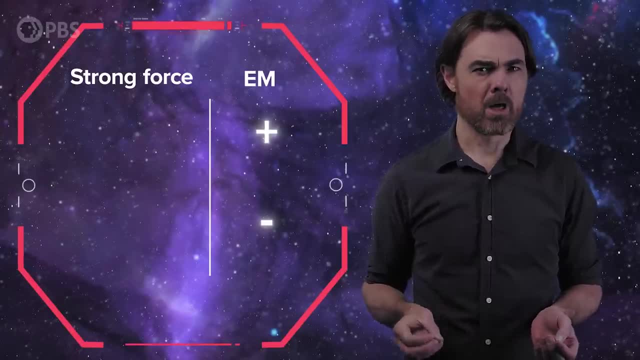 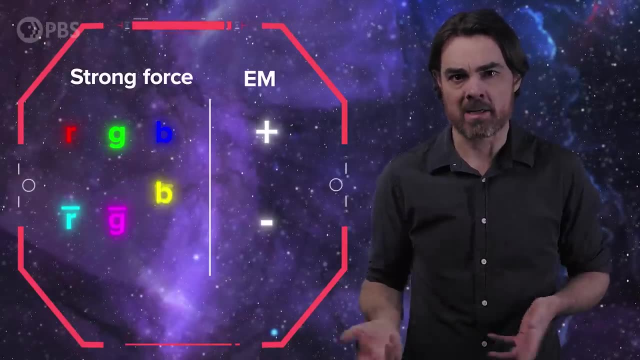 unlike the single type of electric charge, A quark, for example, could have a color charge of red or green or blue, or the opposite color charges of anti-red, anti-green or anti-blue. These names, by the way, are just analogies. 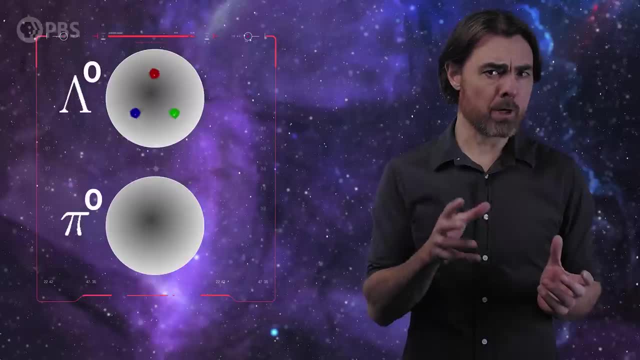 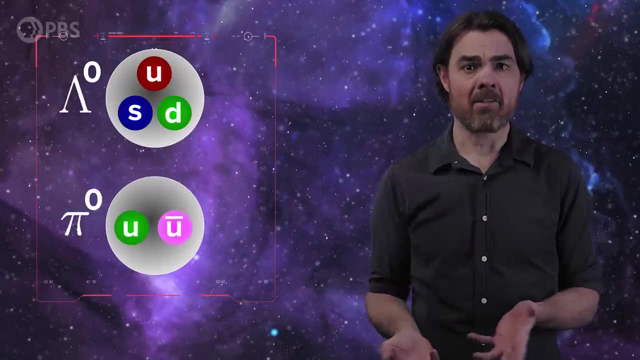 Composite particles need to be color neutral. so the three quark baryons have one of each color charge which cancel each other out, while the two quarks of a meson have a color and its anti-color. These quarks are bound by the strong force which 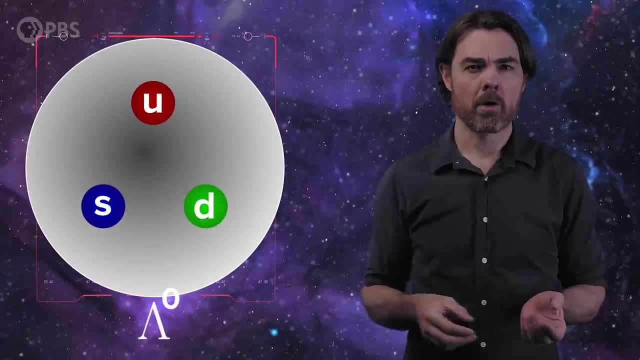 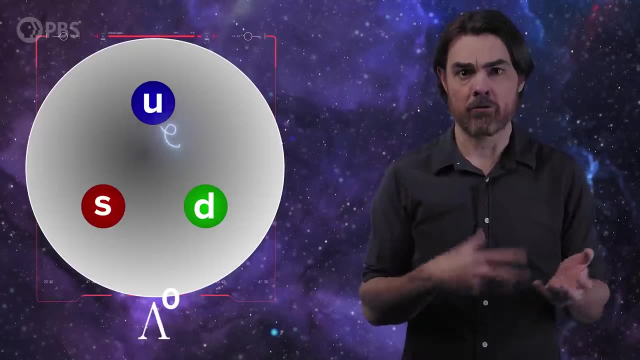 is mediated by a massless particle called the gluon. Gluons each carry one regular and one anti-color charge and they cause the colors of quarks to change. Quarks do flip when absorbed. Baryons and mesons are held together. 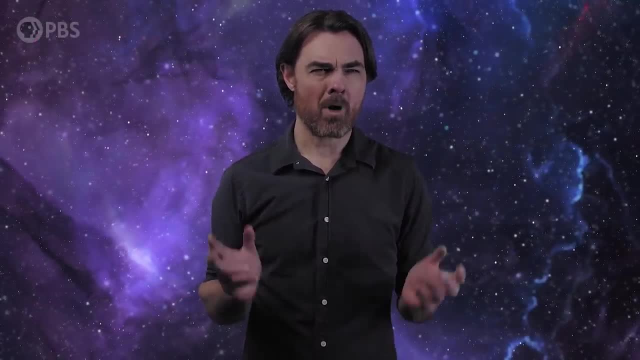 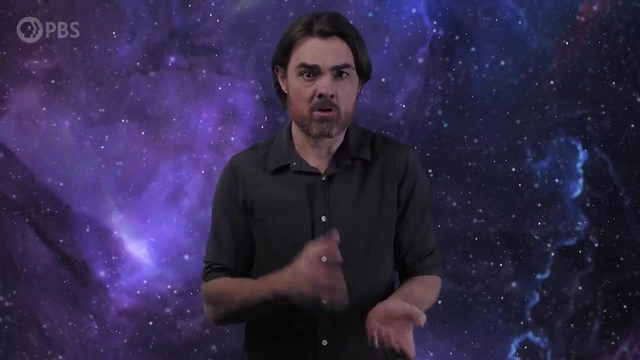 by a continuous exchange of virtual gluons. But wait a minute. Haven't we been saying the entire time that the reason the strong force has a short range is because it's transmitted by mesons with mass? Well, that was Yukawa's whole deal. 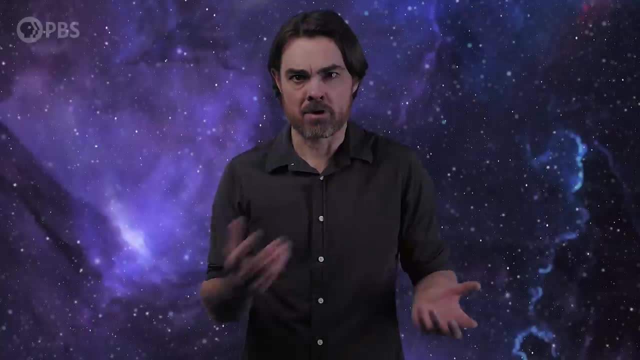 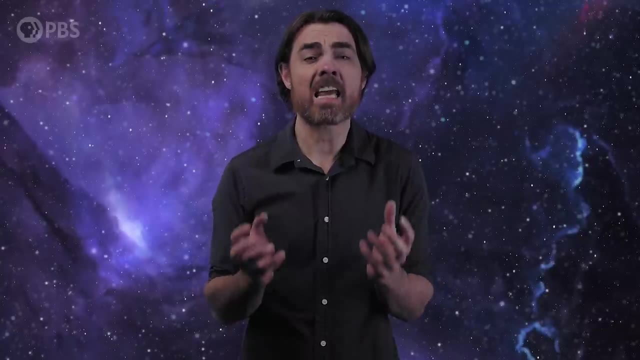 but now it turns out that mesons aren't the real exchange particles of the strong force and the real ones, the gluons, don't have mass. What's going on? Actually, The color-neutral hadrons can't even feel the strong force directly. just. 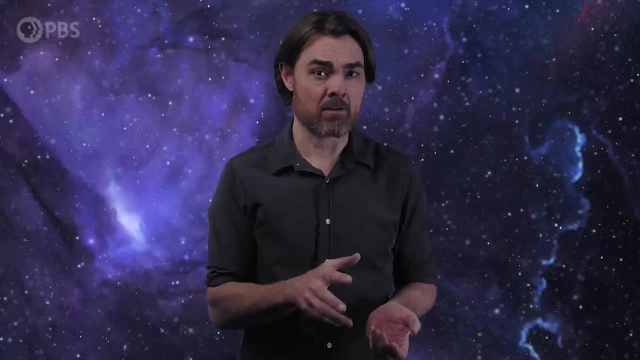 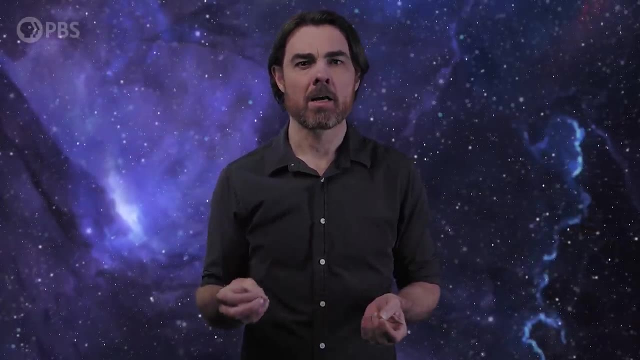 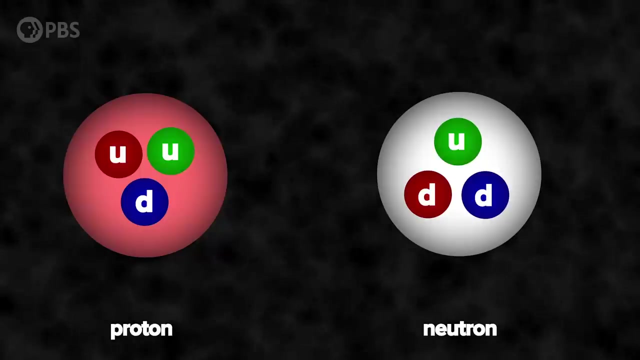 as electrically neutral objects don't exert an electrostatic force on each other. But there is a workaround. Atoms seem electrically neutral from afar, but if you are close enough to the nucleus you would feel its positive electric charge. Similarly, if protons or neutrons 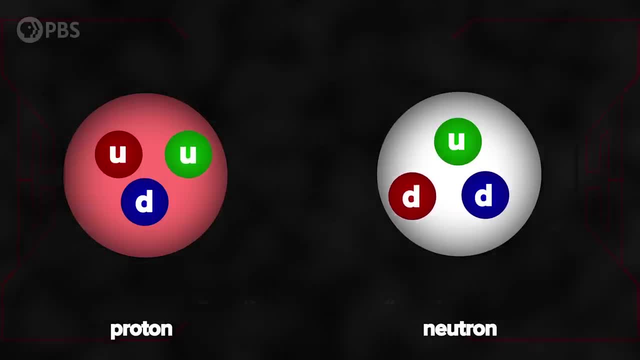 get close enough to each other, their internal quarks will fickle each other's presence. A quark from, say, a proton would, for example, want to tug at a quark from a neighboring neutron, But they can't simply exchange a gluon to do that. 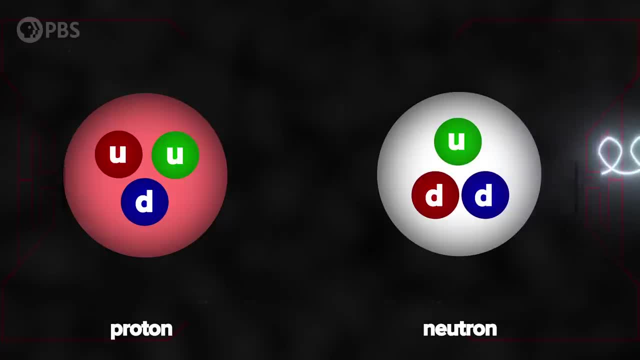 because gluons have color charge, so exchanging a gluon would cause the hadrons to no longer be color-neutral, which is not allowed. In order to properly feel the strong force, the hadrons need to exchange a neutral particle, and nature has found a way to make that happen. 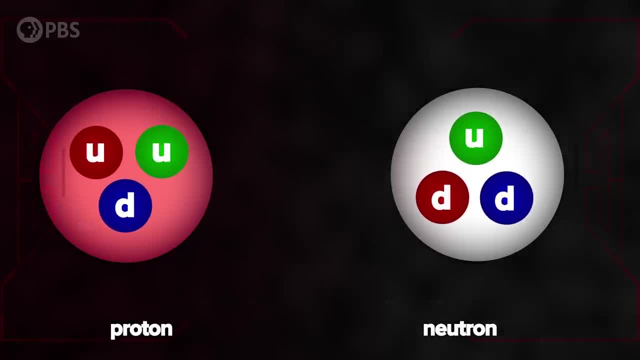 Here's how it goes: A pair of nucleons get close and a quark from one gets pulled towards the other. Its gluon. connection to the other quarks in its nucleus- what we call a flux tube- extends and snaps and in the process generates two new quarks. 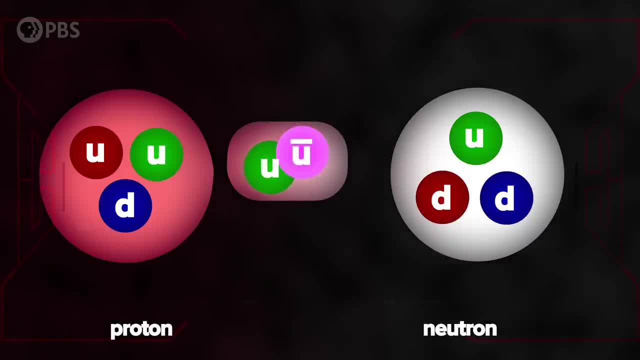 One remains in the nucleus, while the other forms a quark-antiquark pair with the original escaped quark. This is our meson, our pion. It's color-neutral, so it can be absorbed by the second nucleus without breaking any physics. 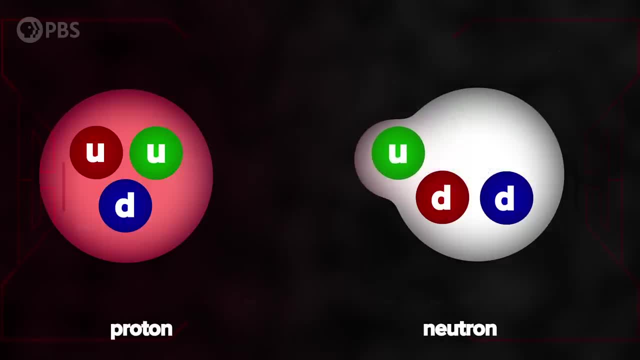 There one of the meson's quarks annihilates with an antiquark counterpart in that nucleus. Ultimately, we're left with two nucleons of the same type that we started with, but they've now communicated the strong force. They did it in a roundabout way, but the process nonetheless. 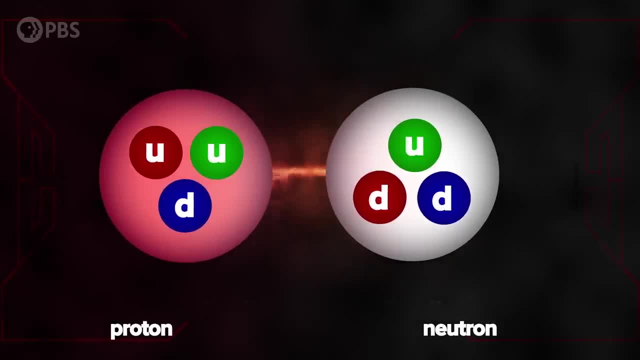 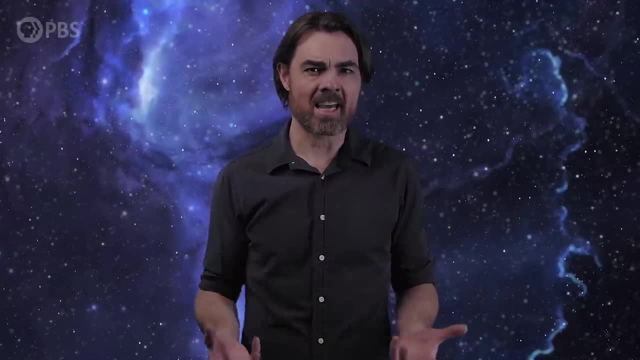 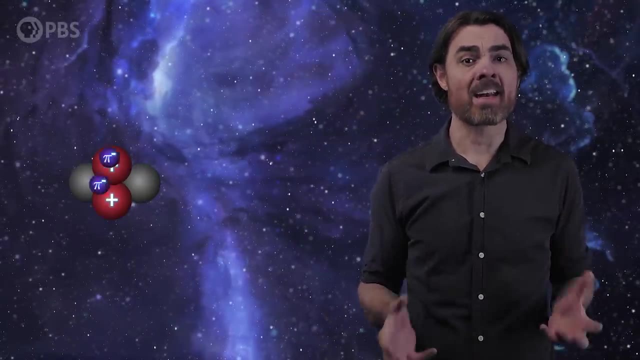 exchanged energy and momentum binding the particles together. This is how the strong force finds its way around its lack of a neutral gluon. It cobbles together a neutral exchange particle, the meson. But the meson has mass. A virtual meson has to borrow a lot of energy. 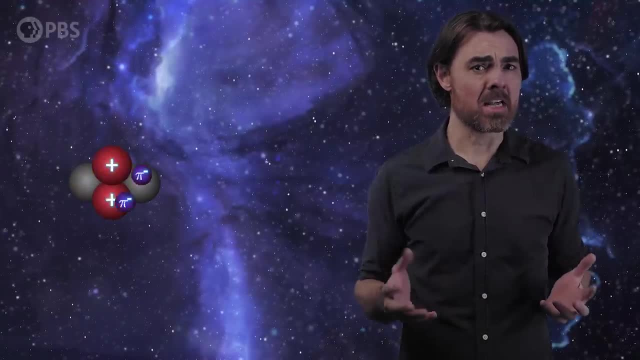 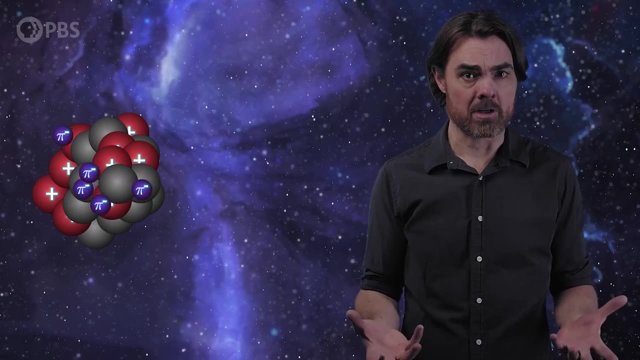 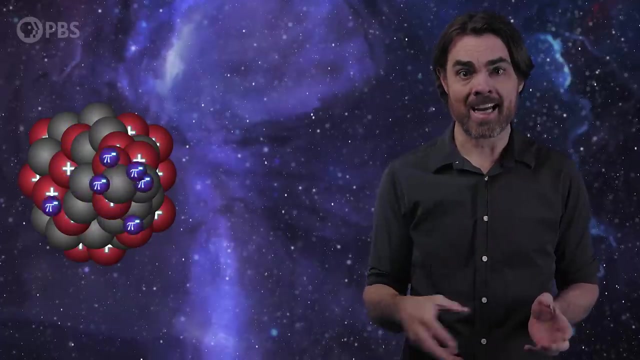 to create its own mass, and so the uncertainty principle says that it can't exist for very long. Its range defines the possible size of an atomic nucleus. If a nucleus gets too big, then its nucleons are too far apart to exchange mesons effectively. 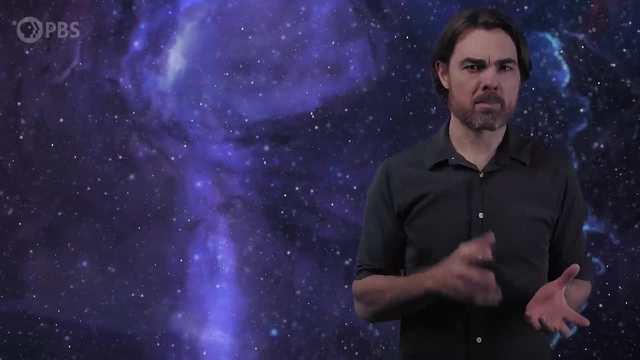 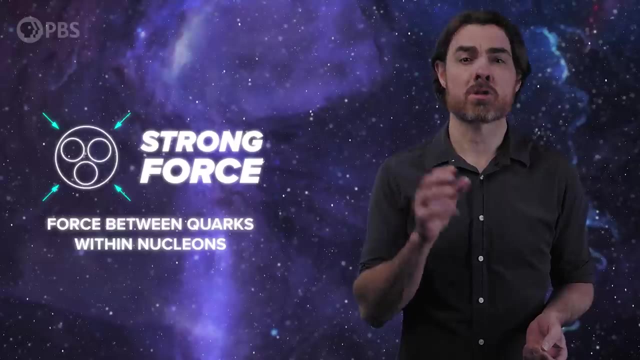 and it'll decay. By the way, when we talk about the force between quarks, we call it the strong force, But this residual strong force that exists between nucleons is called the strong nuclear force. You know, this reminds me of our episode about quasi-particles. 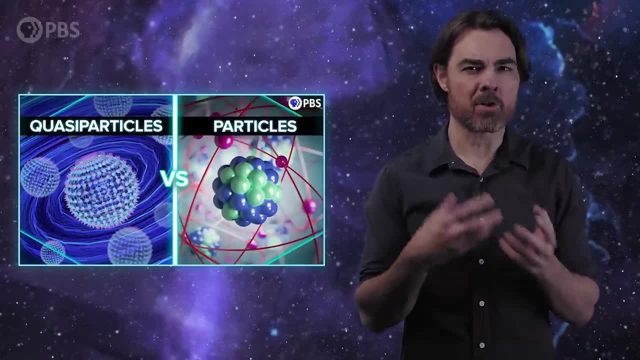 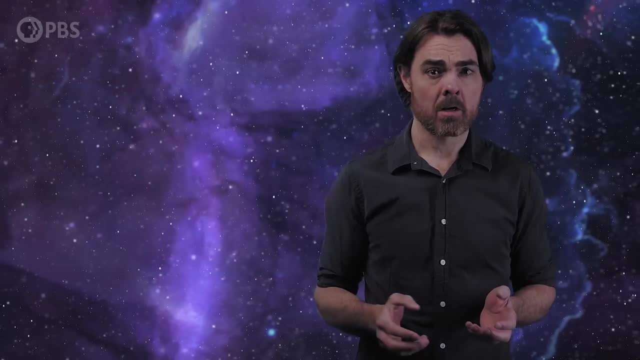 In that episode we talked about how fields can arise as emergent behaviors of other fields, and these quasi-fields will have their own quasi-forces and quasi-particles. Well, that's sort of what's happening here. The strong nuclear force is a quasi-force, mediated. 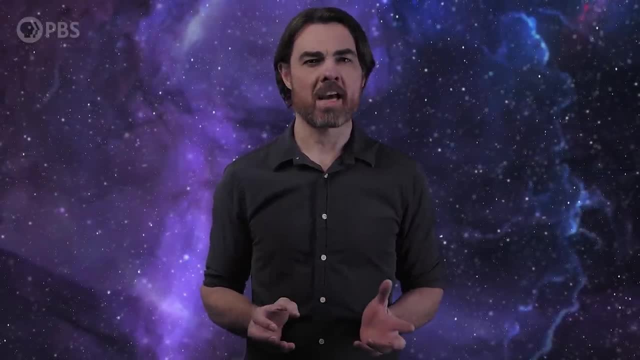 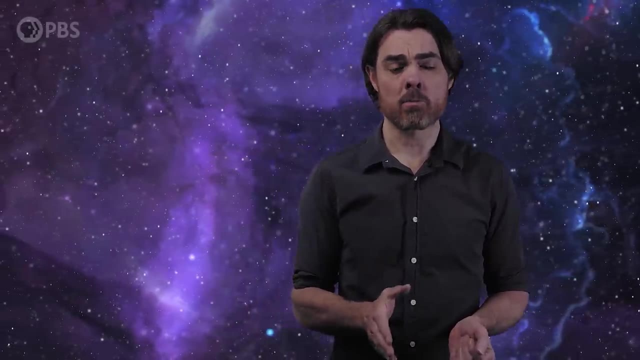 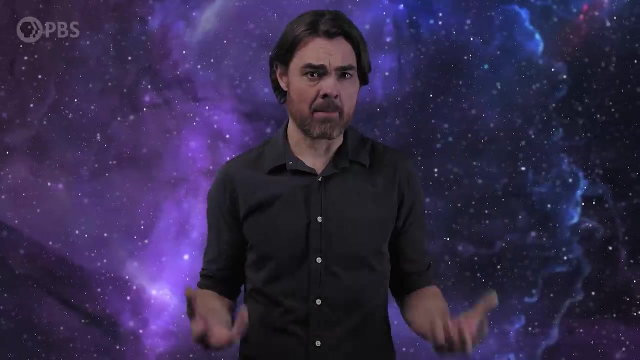 by a quasi-particle, the meson. Without this little quirk of nature, this emergence of a force that's not really supposed to be there, the most complex atom in the universe would be hydrogen. Fortunately, nature stumbled on a way to bind the nuclei, which gave us chemistry and biology. 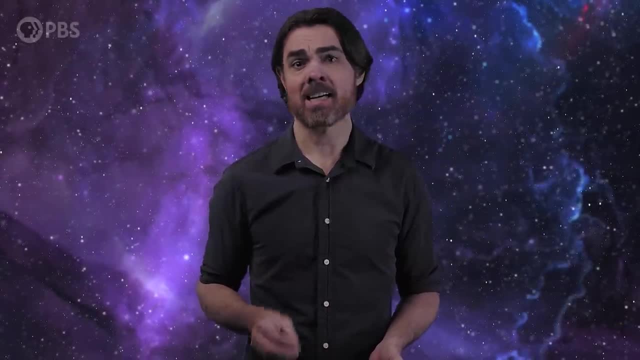 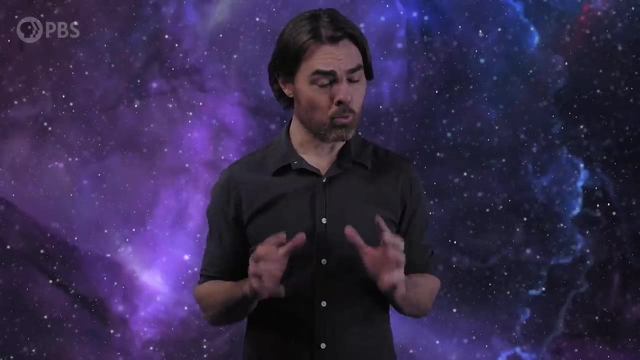 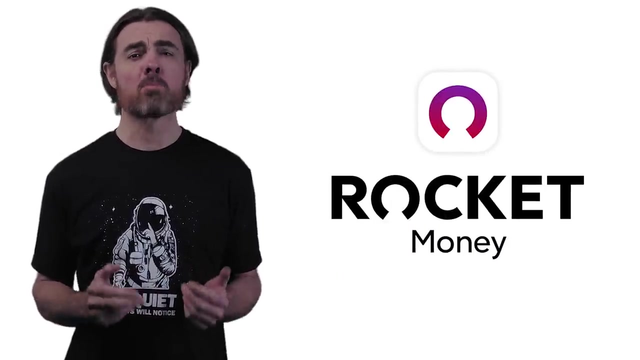 and ourselves, including a young physicist named Hideki Yukawa, who was able to figure out some of the most important forces from which emerges this richly complex spacetime. Thank you to Rocket Money for supporting PBS, Because life only gets more complex and complicated, busy and expensive.